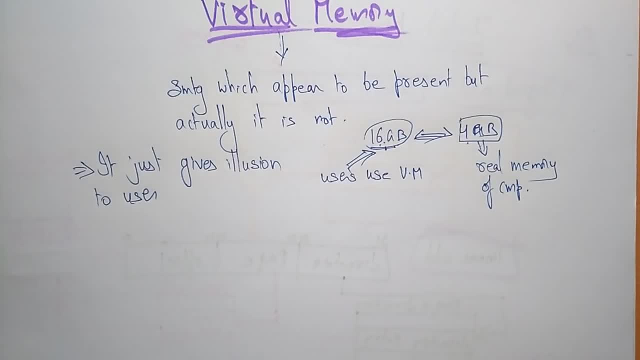 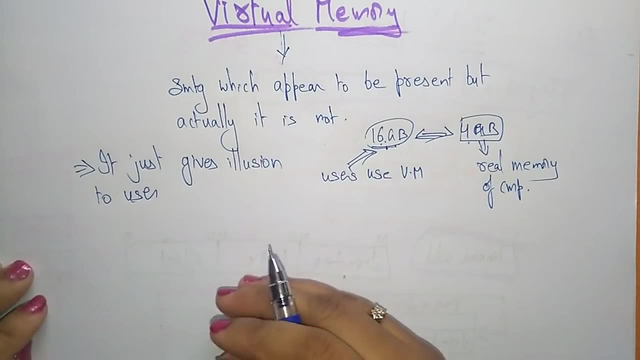 So just it gives a illusion that they will have main memory equal to the capacity of secondary storage media. So the programmer can write a program which requires more memory than the capacity of virtual memory. Actually, whatever the programs we are writing, So that 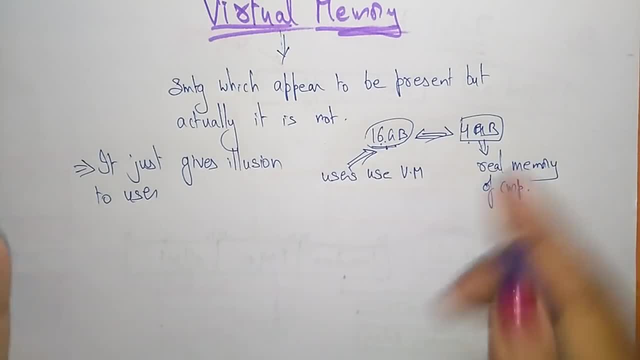 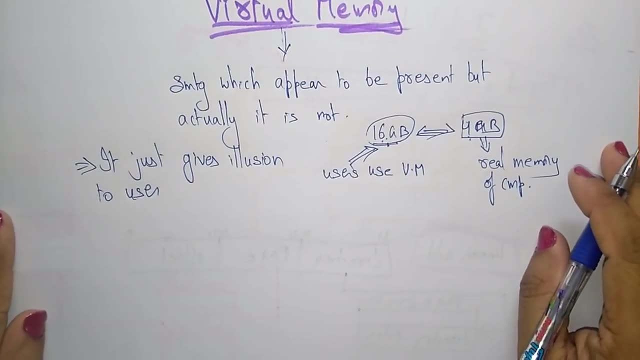 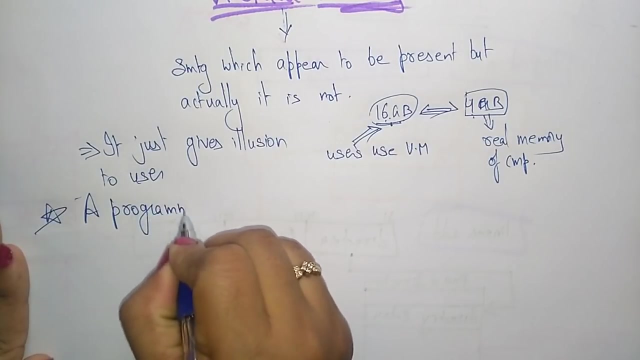 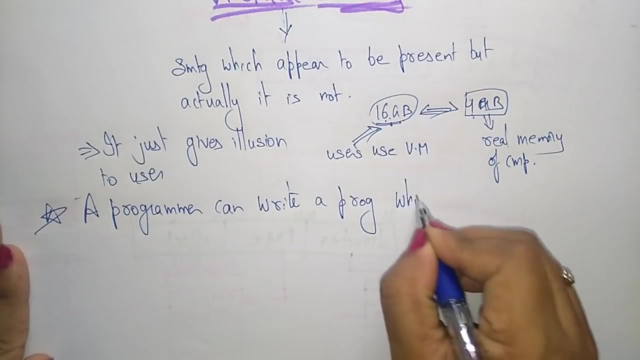 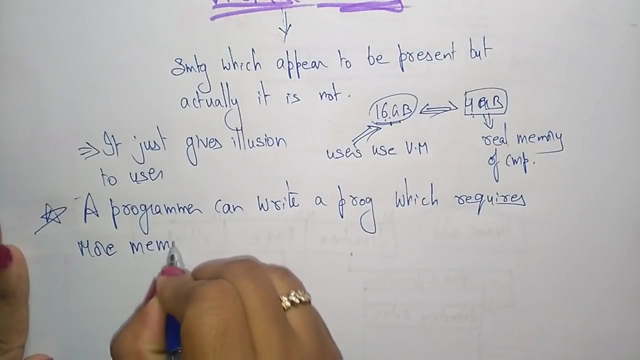 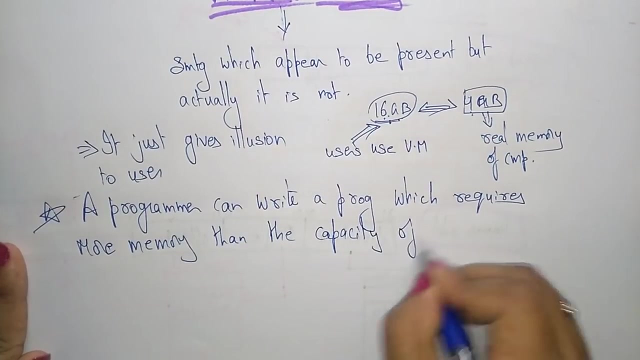 That programs requires more memory than the capacity of, than the capacity of main memory. So such program is executed only by virtual memory technique. So let me write that point: A programmer can write a program which requires more memory. So the programmer can write a program which requires more memory than the capacity of main memory. 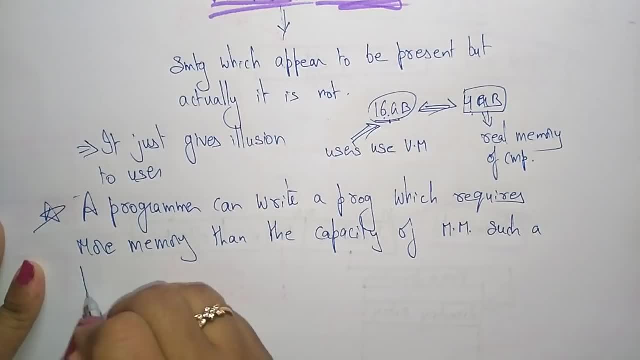 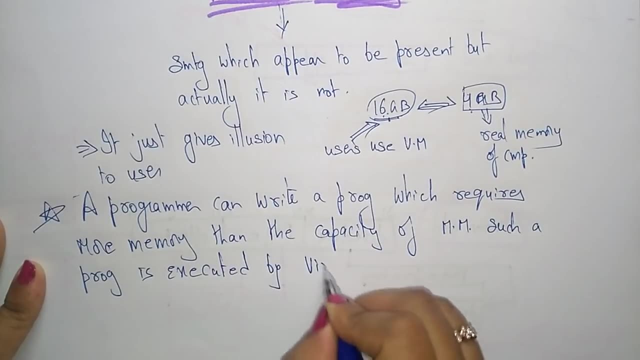 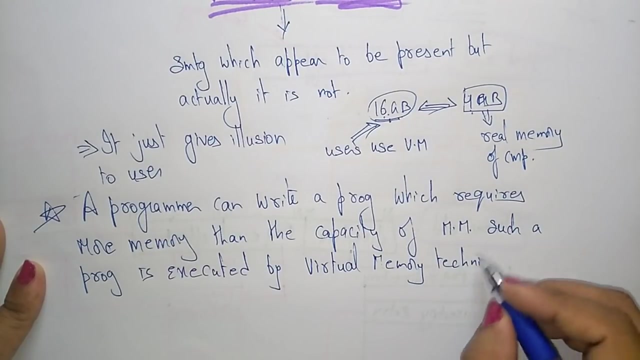 Such programs. Such a program is executed by virtual memory technique. So with the help of the virtual memory technique, Those programs will be executed. Those programs will be executed, execute in main memory, so we can say that primary memory, or the main memory, or the physical memory, 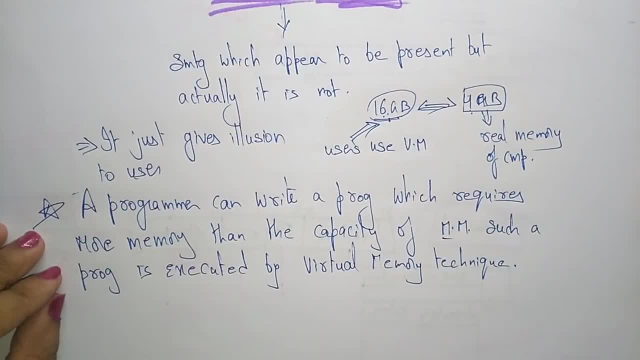 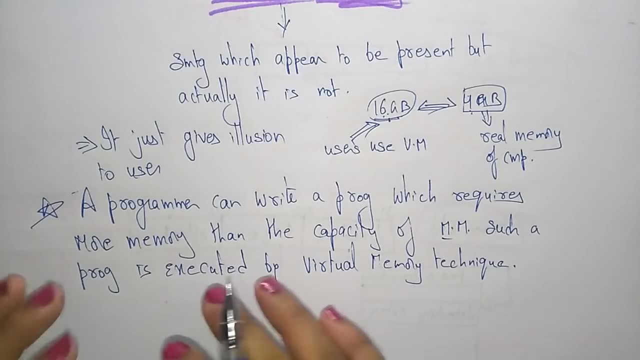 everything. this is a finite, so only the finite, whatever we are using. suppose it is a 4 gb or 16 gb or 18 gb, so like that- so that will be a finite, whereas virtual memory is infinite. so you can use uh how much you want. the programmer requires uh how much the memory he want he can. 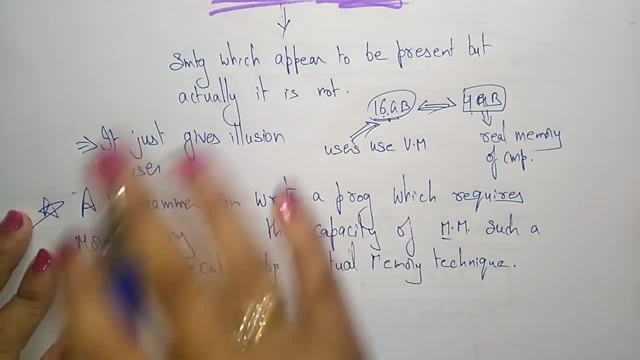 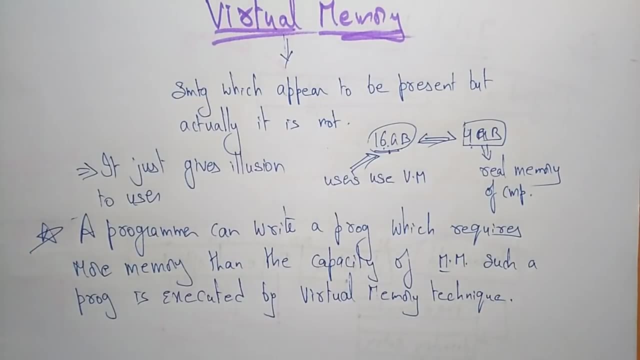 use. so it is not a constant. virtual memory is not constant, whereas the main memory is a finite. okay, so, uh, so, because this is just an illusion to the user, it actually doesn't appear, but we thought that it is appear. so that is a basic introduction about the virtual memory. so the virtual memory is 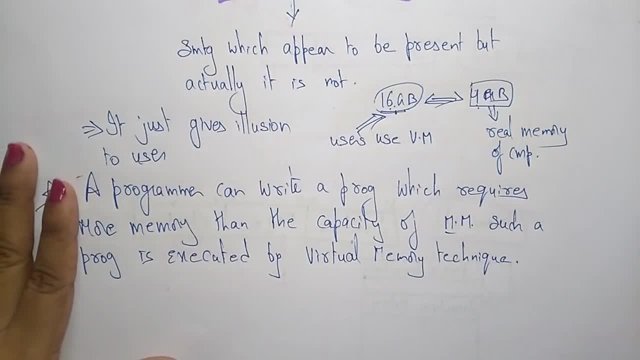 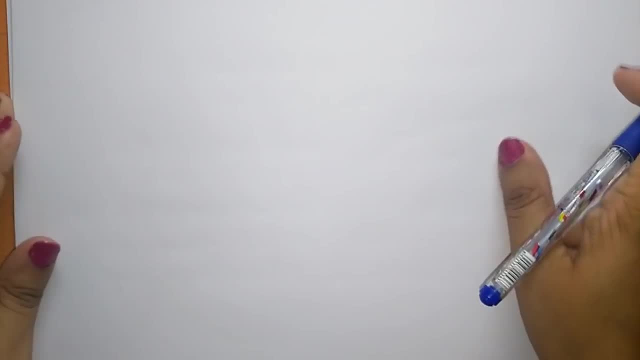 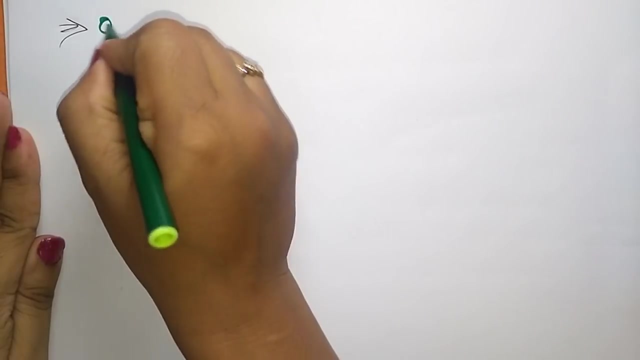 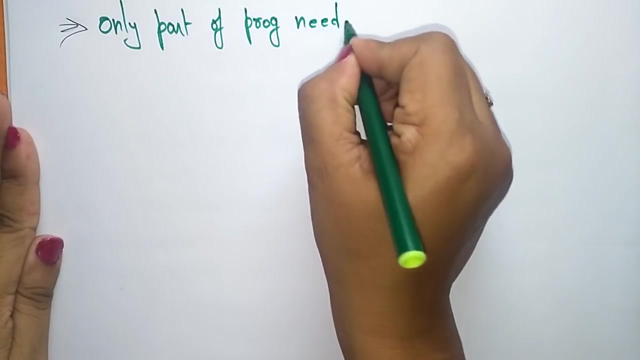 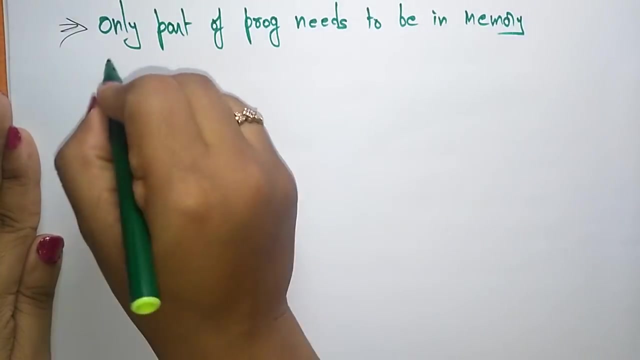 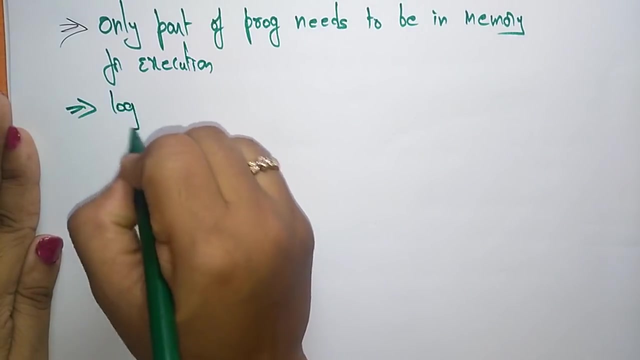 a separation of user logical memory from physical memory. so let me write some points regarding this virtual memory. let me write these points. virtual memory, uh, only part of program. part of program needs to be in main memory for execution, to be in memory for execution, execution. so the then logical address space. 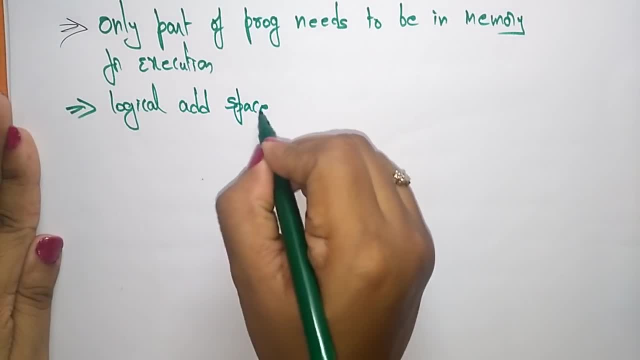 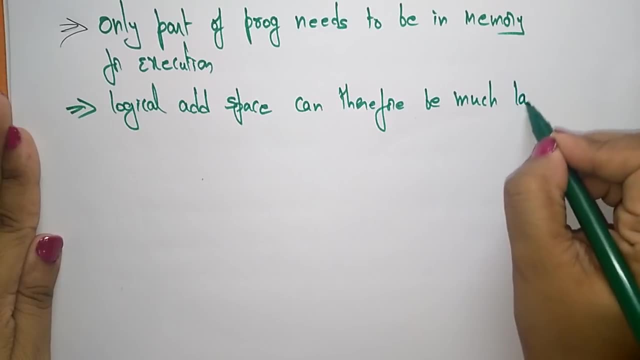 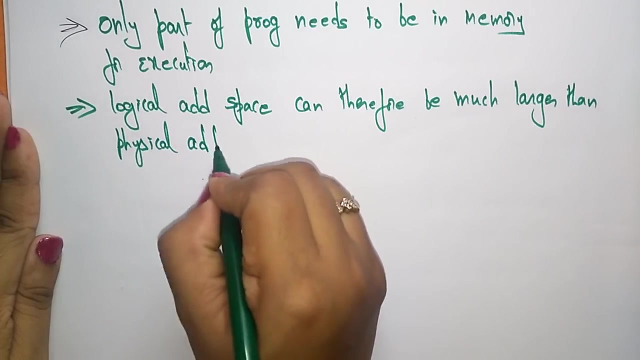 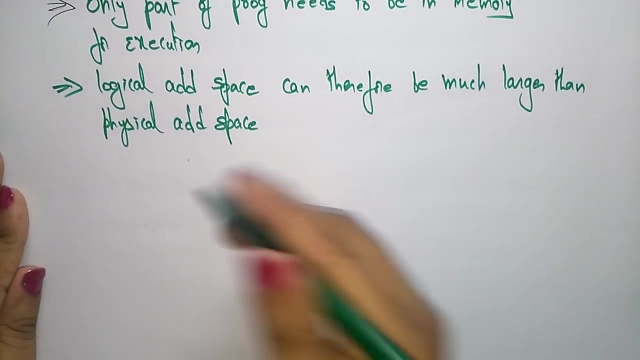 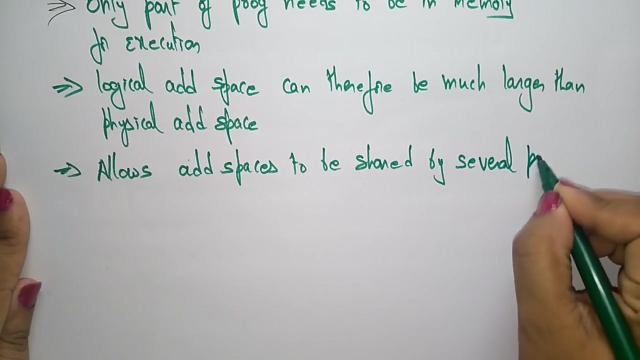 can therefore be much larger than physical address space. so, whatever the virtual memory that is a logical address space we we are using, that is much larger than the physical address space. so then, allow address space. allows us address spaces to be shared by several process, by several processes. 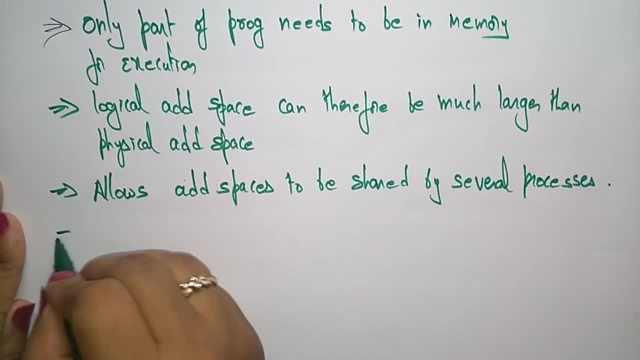 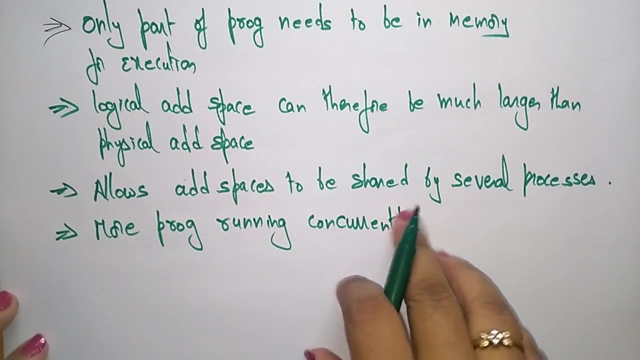 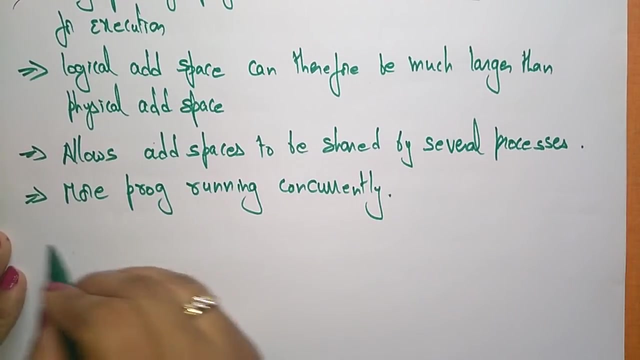 and then more programs, more programs running concurrently using this virtual memory technique. so this virtual memory uh can allows address spaces to be shared by several process and more programs can run concurrently by using this virtual memory technique. So it requires this virtual memory requires less I-O need. input output need is less to load or even to swap the. 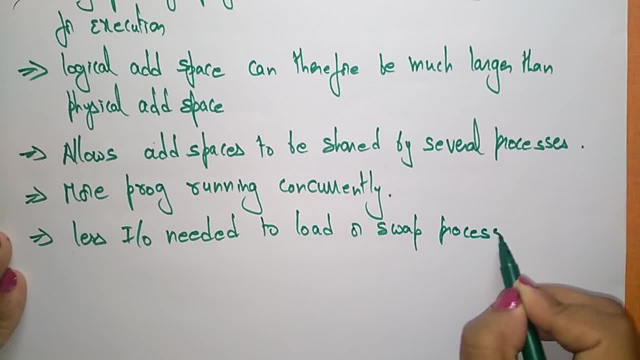 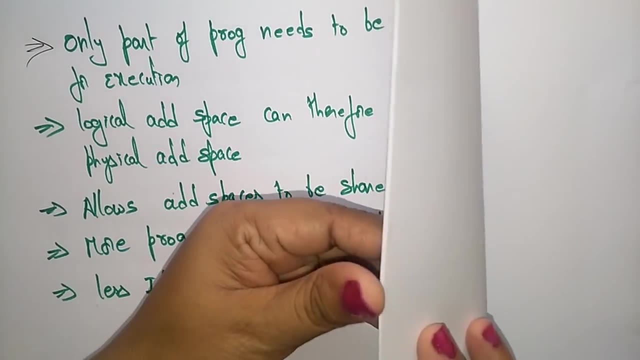 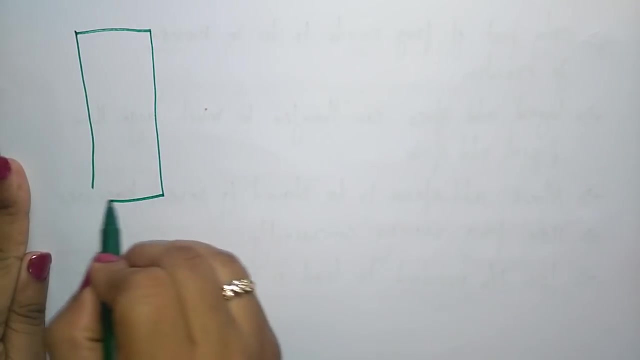 process, So to swap the process or to load the process. this virtual concept uses less input output requirement. So let me explain with simple example how this virtual memory is dealing with physical memory. Let us take this: is suppose this is a virtual memory, So virtual memory is also. 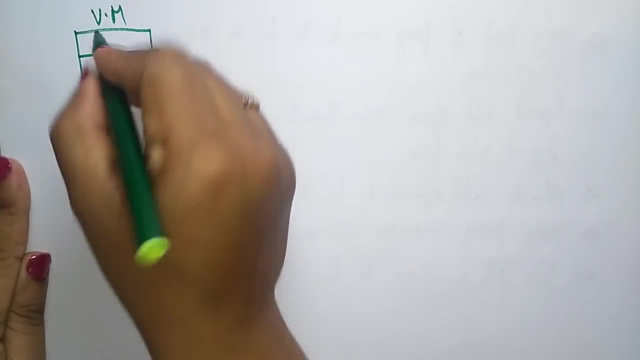 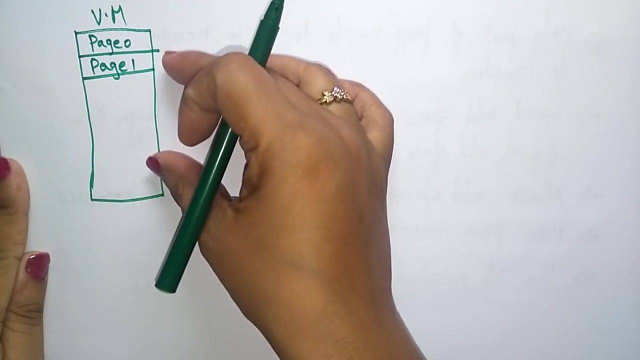 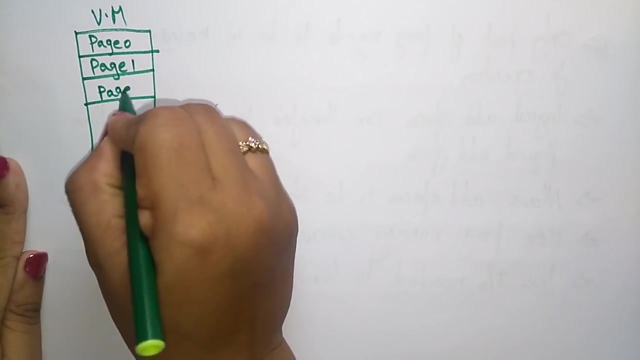 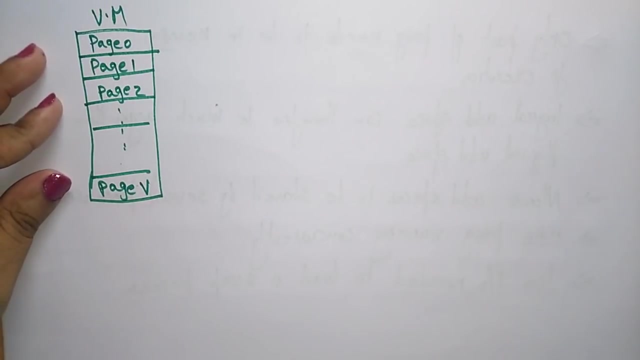 called as logical memory. This concept I already explained. So let us take the page 0, page 1.. So the virtual memory always uses the concept pages, whereas a main memory, that is, a physical memory, uses a concept of frame. So page 1, page 2, so up to page 3.. So let us say this is a virtual memory and here we are taking 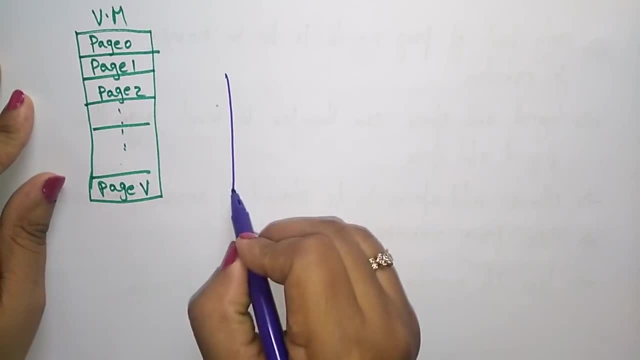 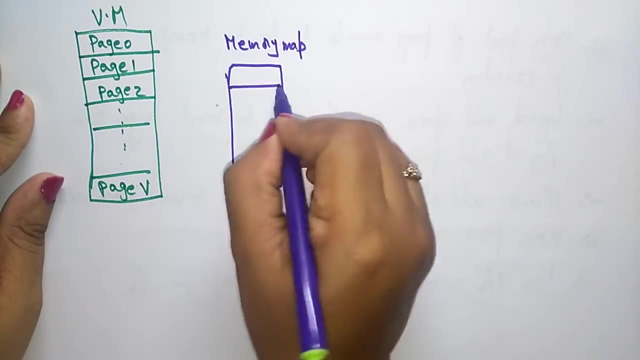 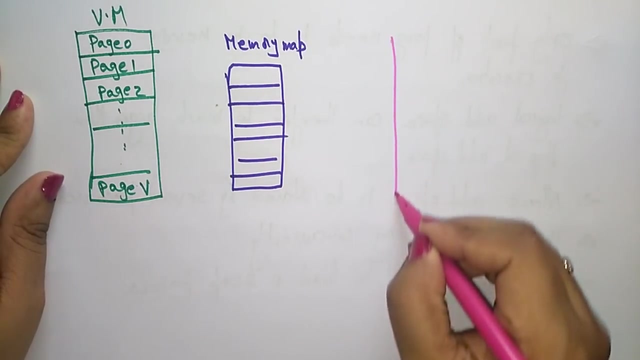 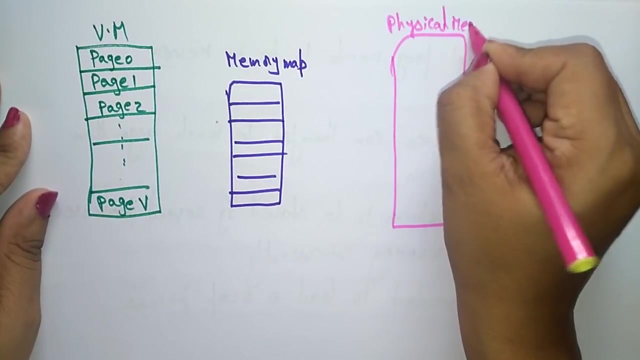 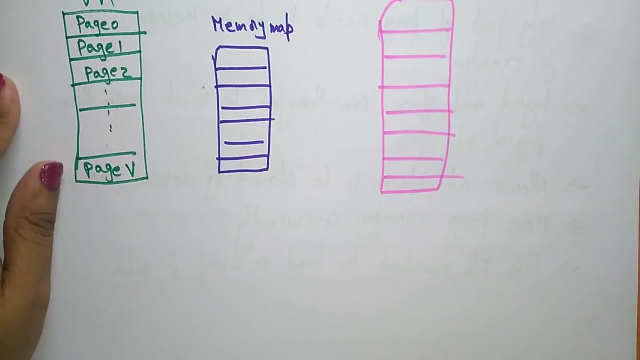 another memory that is a memory map. So with the help of the memory map, we are pointing to the main memory. So this is a memory map, and then it is having the physical memory, And this is the physical memory, and then it is having the disk. that is a secondary memory.